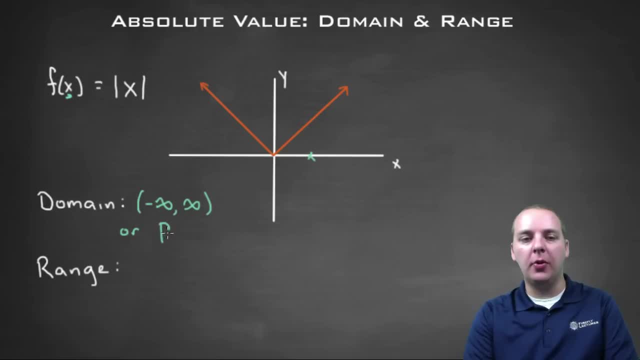 with Uh. or you can write a capital R with an extra bar out front. That's math shorthand for the words all real numbers, Basically saying your domain is all x values, Um. or you can write it out in English. You can write the words all real numbers, Alright, so usually any. 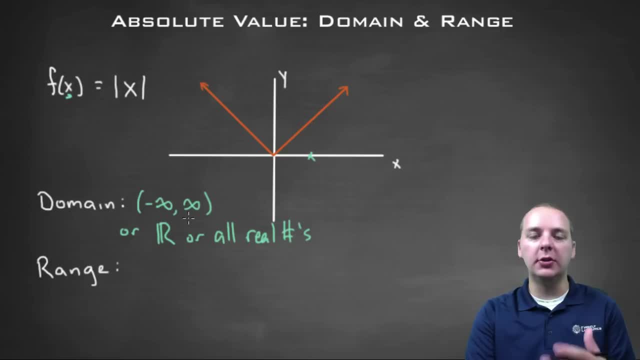 of these would be acceptable. You just might want to check with your instructor just to make sure you're writing it how they would prefer If they would rather interval notation or something like that. Alright, um, now what about range? Range is a little trickier, though. 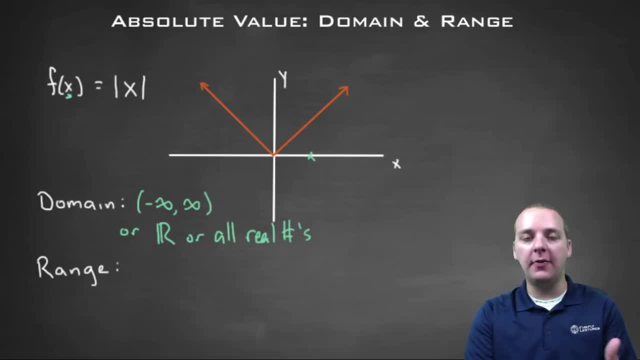 The range is the y values, that the set of y values that come out of the function. So if it's just an absolute value of x function, well the y values you would get out would be zero and greater. You can't get a negative out of a, out of an absolute value, uh term. 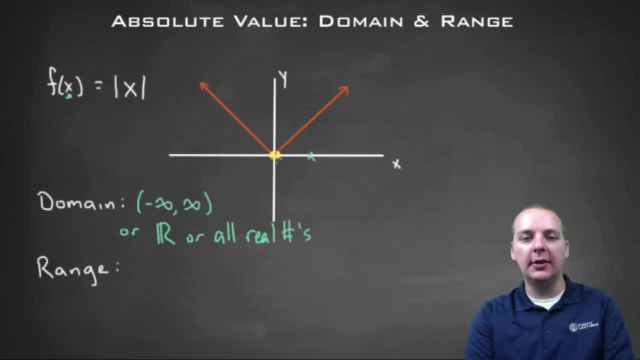 like this. So it looks like our y values that we get start at zero and then go up to zero And then go upwards from there. So our range would be either from zero to infinity, if we wanted to use interval notation, Or we could say all the y values that are greater than. 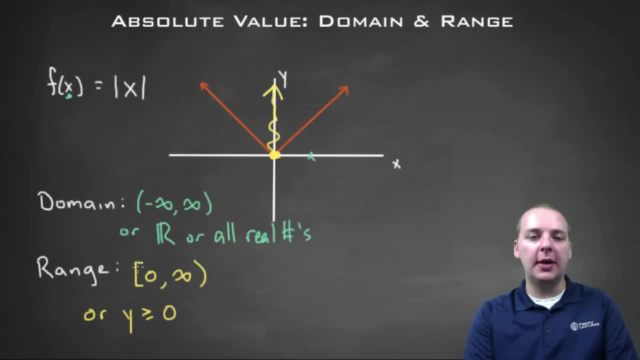 or equal to zero. Either way is fine. And notice, I put a bracket around the zero because we actually do get this y value. But any time you have an infinity in interval notation you're gonna put a, a parenthesis there, Alright, so this is the interval notation And the 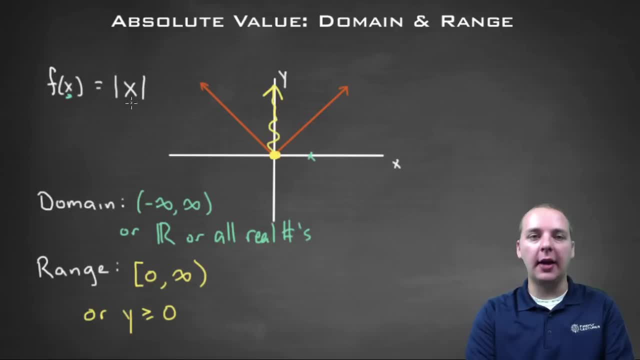 y values that are greater than or equal to zero. this is the domain and the range of just the, the generic absolute value graph. Now, this is probably not what you'll have on your homework and test. Um, what you'll probably have is some version of the absolute. 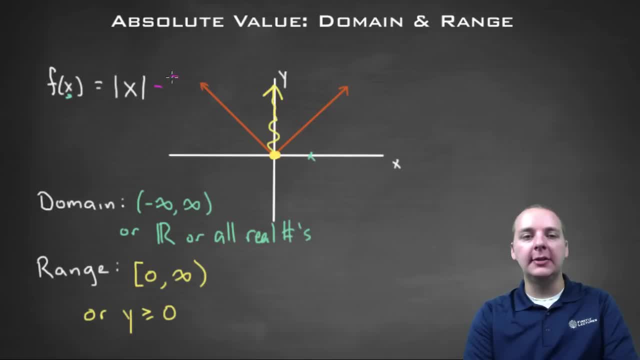 value function Like the absolute value of x minus five, You know, or something something like the absolute value of x plus two um plus ten, You know, or something like that, where the uh generic parent function: the absolute value of x minus five, you know. 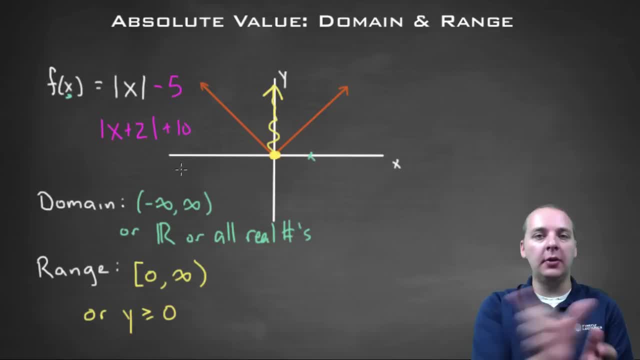 the absolute value. v-shaped graph is moved up down, left or right, Possibly reflected And, depending on how advanced your course is, maybe even stretched or compressed, Which will even change the steepness of it a little bit. So what? what would change if you had?